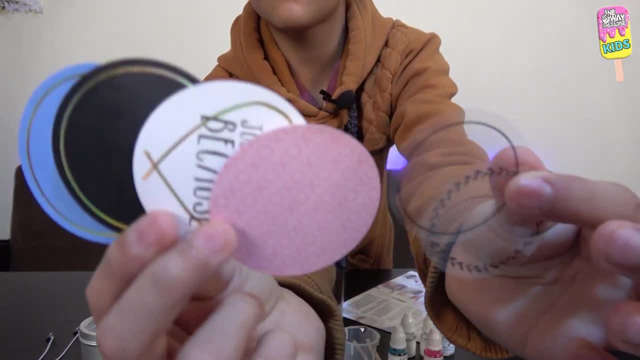 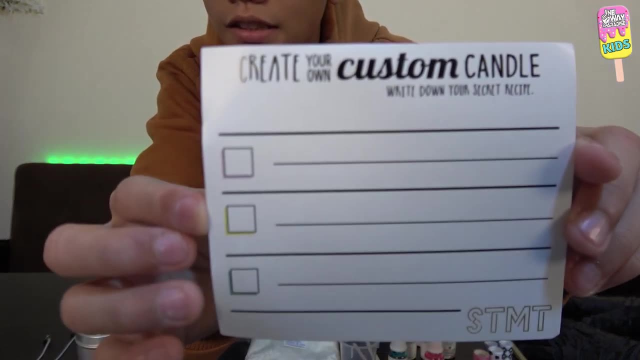 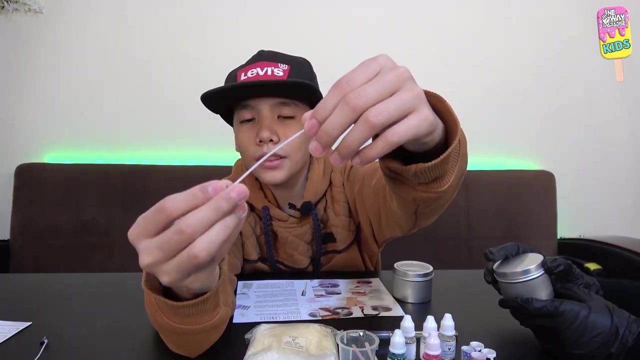 some fragrance droppers, liquid dye, some labels, some stickers to wrap around the tin cans, a gel pen and, last but not least, a recipe card. So the first step to make our candle is to get our tin cans and we will get the waxed wick and we will get a glue gun and put some glue on the end, right. 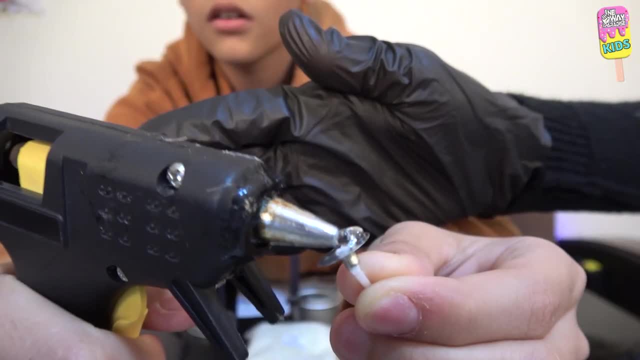 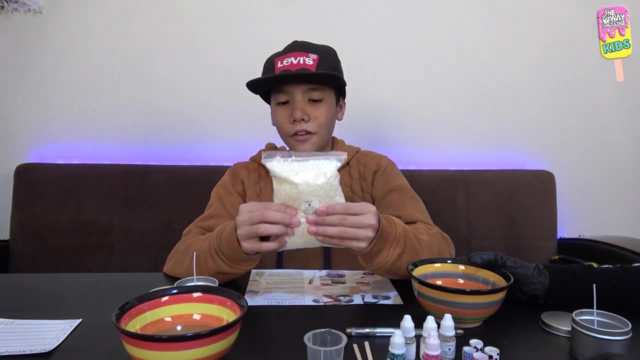 here and place it in the middle. We will just demonstrate. The next step is to get our wax chips and we will get half of it and fill it in the bowl. So our next step is to make our candle. So we have our waxed wicks and we will get some glue on the end right here and place it in the middle. We will just demonstrate. 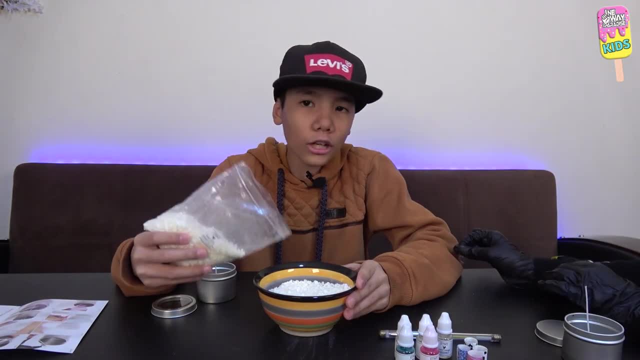 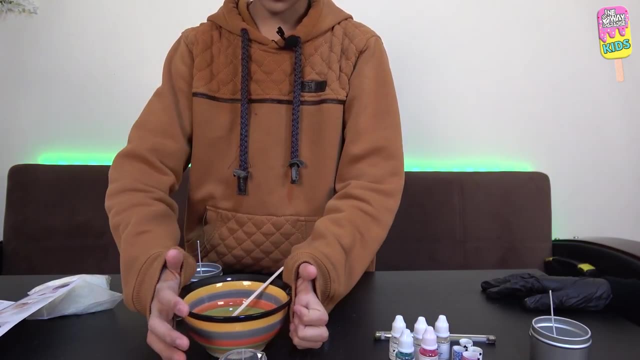 The next step is to get our wax chips and pour half of it into a microwave proof bowl, and we will put that in the microwave for three to five minutes. Okay, so we just microwaved it for three minutes and 30 seconds, and it is now a bit liquidy. 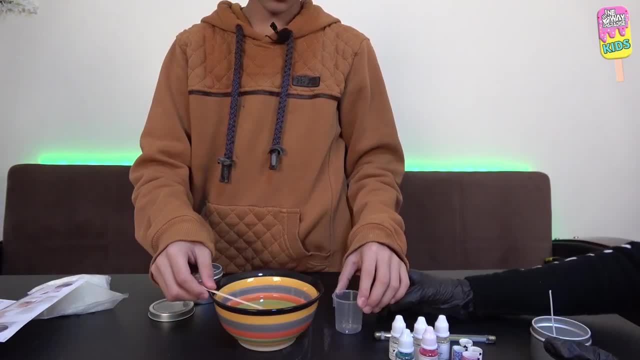 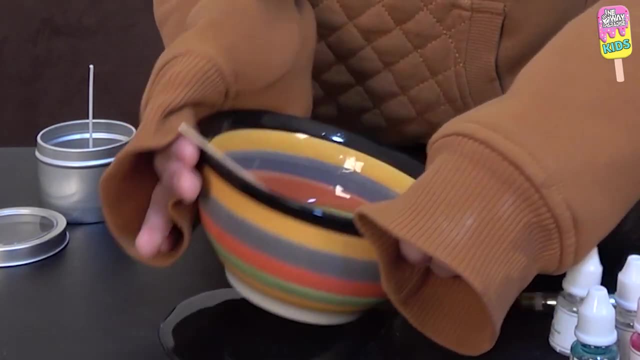 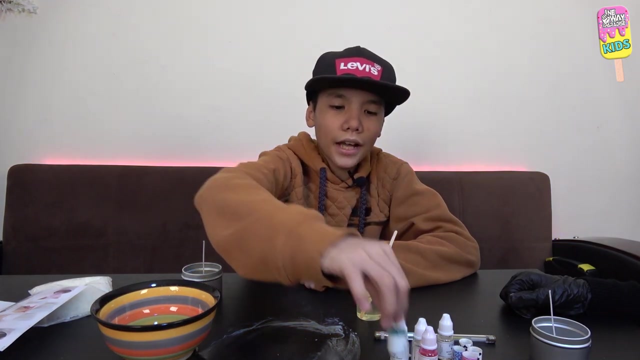 So we're going to have to work fast. What we will do is we'll get our bowl and pour it up to 30 milliliters. What? okay? so we made a little mess because it rolled down the bowl, but now we'll just pick our color. 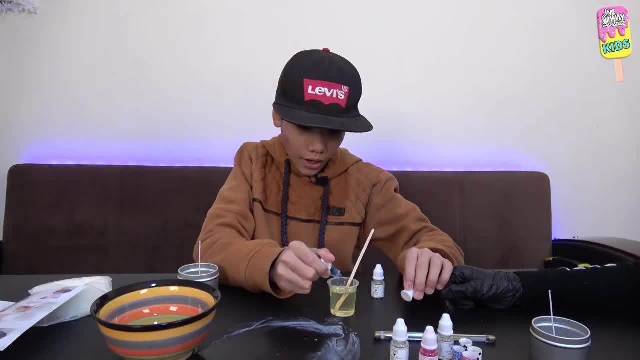 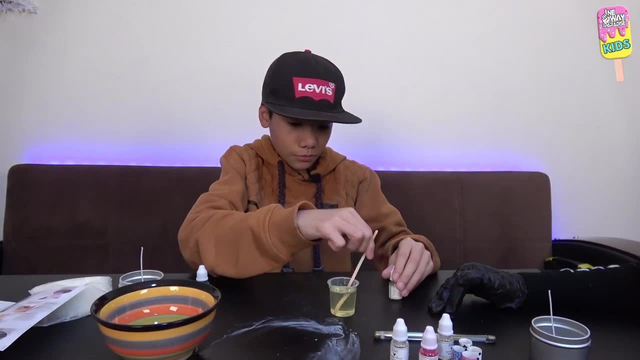 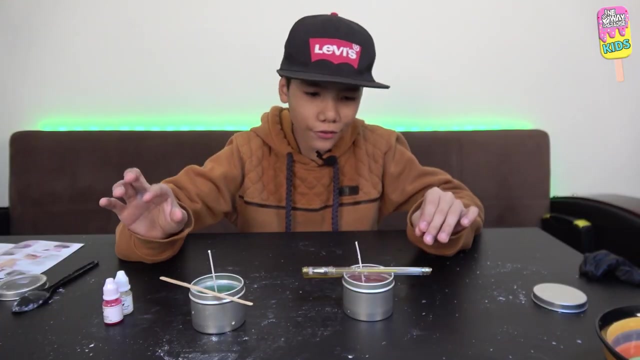 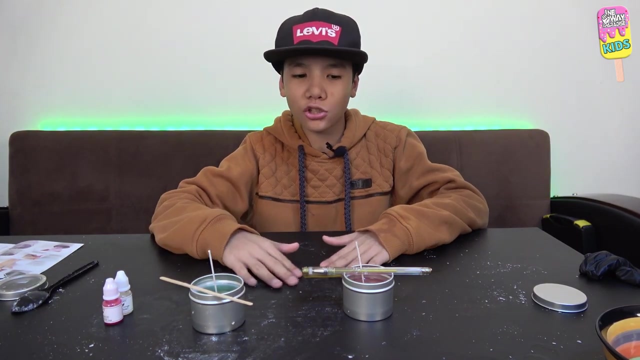 and fragrance and we'll just pour it into the wax. i'll just pour three of this and i will get rose and and i'll just mix it and now we just pour this into our tin can. we just finished filling our tin cans with candle wax. just a quick heads up: make sure you use a tray. 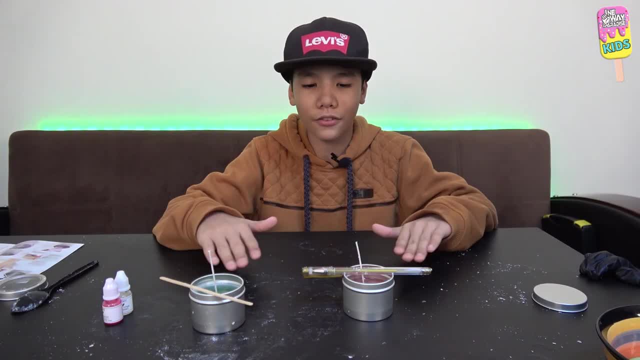 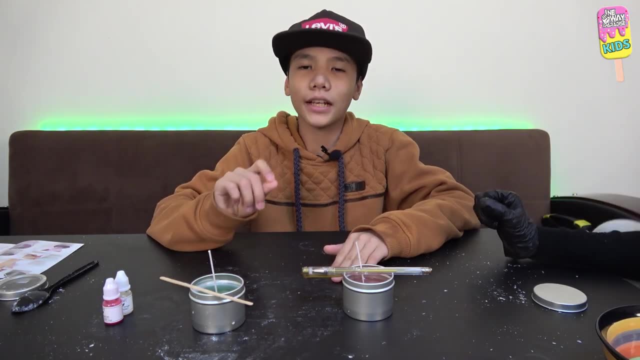 or something, before you pour in the wax or do any of this, because i don't know if you can see, but we made a big mess and the wax spilled all over. so that's just a quick heads up, uh, but now all we gotta do is wait for half an hour, and it should be dried by then, inshallah. 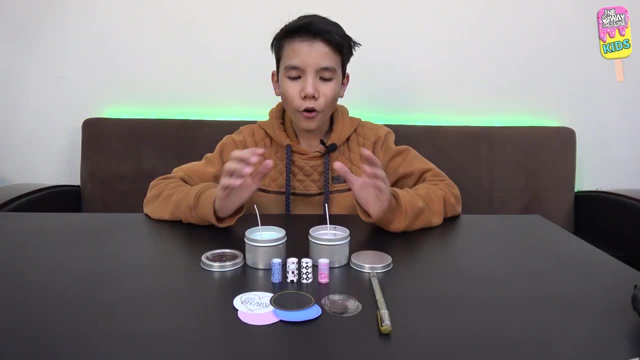 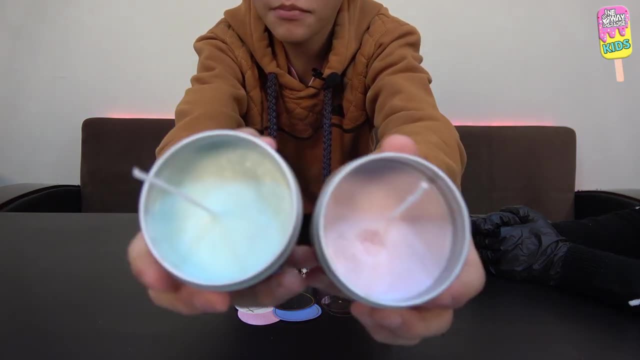 okay, so we're back. we let our candle wax sit for 30 minutes, and here's what it looks like for 30. after 30 minutes it's all dried up and nice. the blue one is mine and obviously this is my sister's, the pink one: